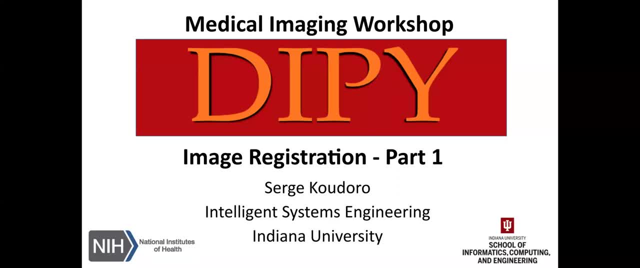 Hello everyone and welcome to DiPi workshop. Today I will be presenting image registration, which is a common step in the medical imaging field. Image registration is in all diffusion imaging pipeline, so I don't see how you can escape it, this step. I know that image. 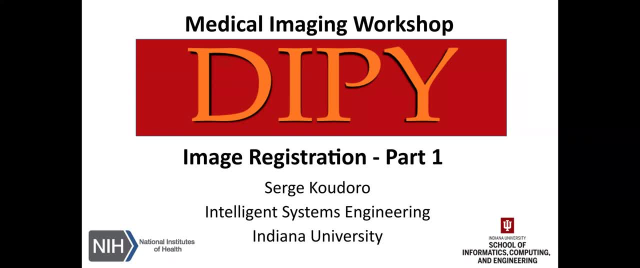 registration is a black box for many people and looks scary. So the goal of this talk is to open this black box and understand all the basics concepts. My name is Serge Coudoureau and I'm a software engineer for the Gary Falidis research group. Also, I'm one of the DiPi. 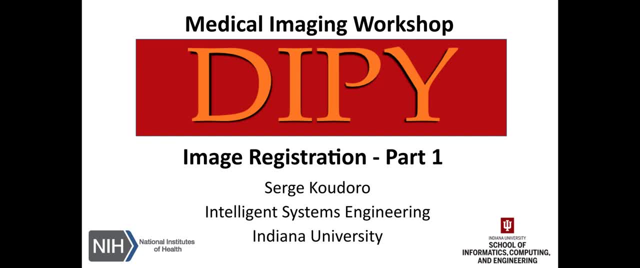 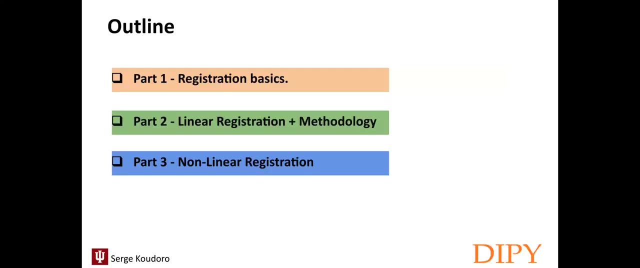 and Fiori core contributors. I'm taking care of the DiPi and Fiori releases and everything related to the maintenance of the BOSS project. So let's start. This session will be split in three parts. The first video is a part one. We will look at the basic concepts of 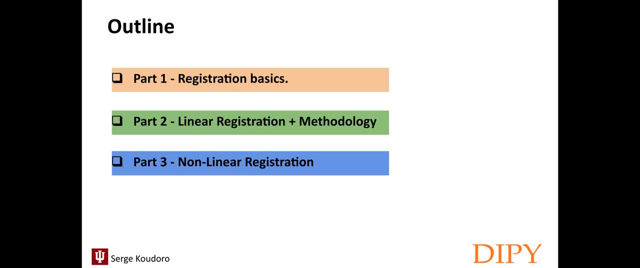 image registration. What are medical, What are the medical acquisition issue And how image registration can solve those problems. In the video two it will be dedicated to image registration methodology and affine registration From transformation to optimizer and including metrics. we will decompose every. 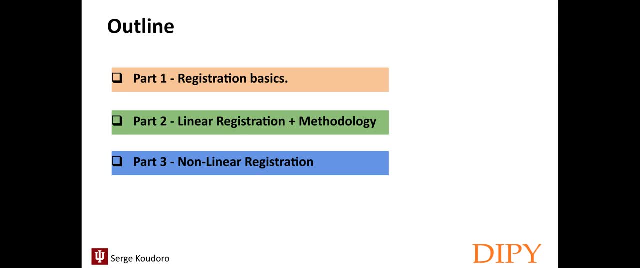 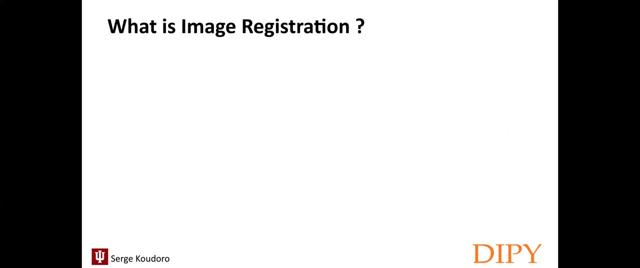 step of the registration process and see how we can use it with DiPi. In the part three we will review some advanced transformation model and specifically the diaphragm orchestration model. What is image registration in medical imaging? So image registration is just an alignment problem. In this simple, simple example, we 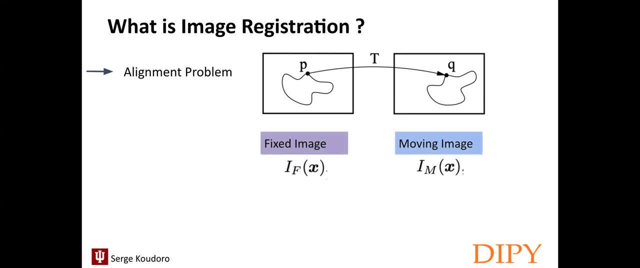 have one moving image that we will call IM the X, that will be deformed to fit the other image, the fixed image that we will call IF the X. To do that we need to find a displacement that we will call D the X. 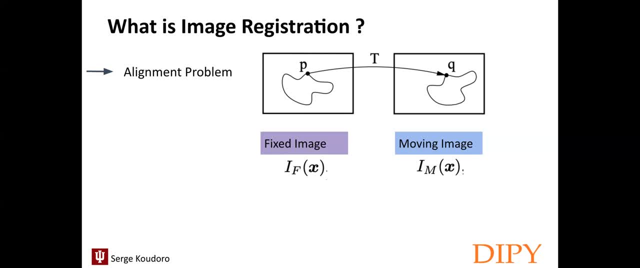 That makes IM the X plus D the X, specially aligned to IF the X. So in other words, an equivalent formulation is to say that the registration is a problem of finding a transformation: T- the X, where you see the equation in this slide. That makes IM. 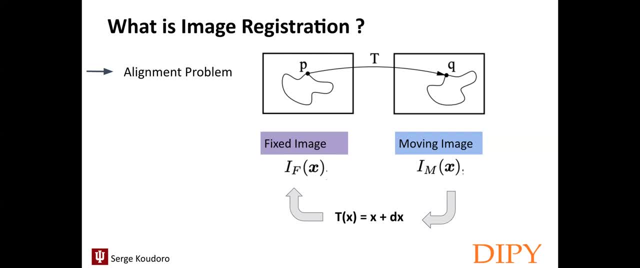 So how, Moving on? We have a fixed image specially aligned to our fixed image. The transformation is defined as a mapping from the fixed image to the moving image, So our goal is to find the best T, the X. Usually the fixed and moving image have a specific dimension, D, and each of the images have their own spatial domain. 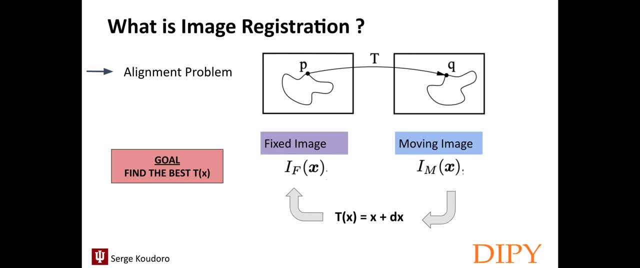 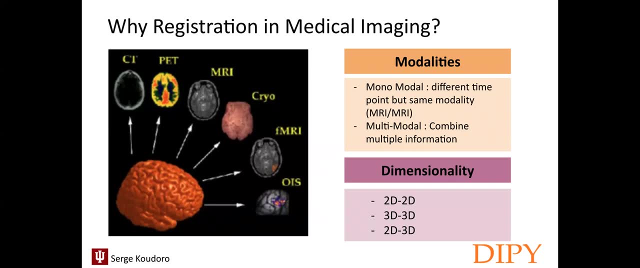 But before we go deeper into that, let's see why do we need this alignment? The first reason is the variety of modalities and dimensionality in medical imaging. A subject can have a scan at a different period of time And you might want to compare them. 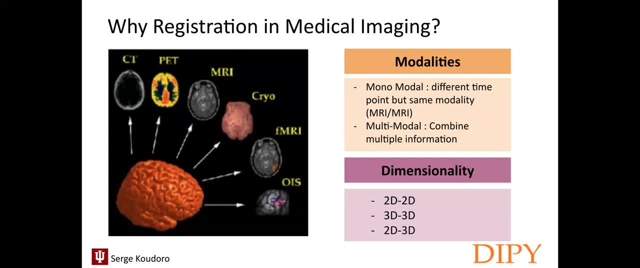 For this task. For this task, You need to align your data, whatever the dimensionality you use, Meaning if you have a 2D slice or if you want to compare a 2D slice with a 3D volume or 2D image or a 3D image. 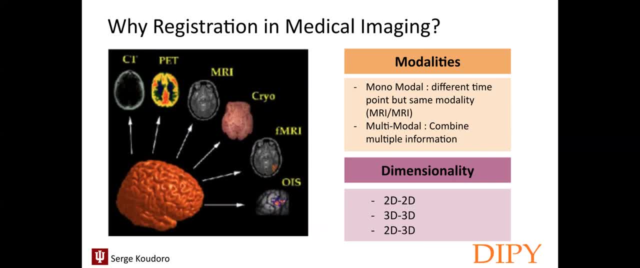 Same story with modalities. Different type of data can be obtained in medical imaging, like CT, PET, MRI, cryo, FMRI or OIS. Aligning different modalities might help you to combine some of the modalities of some of them. 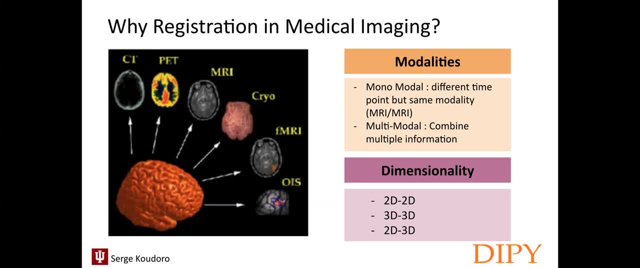 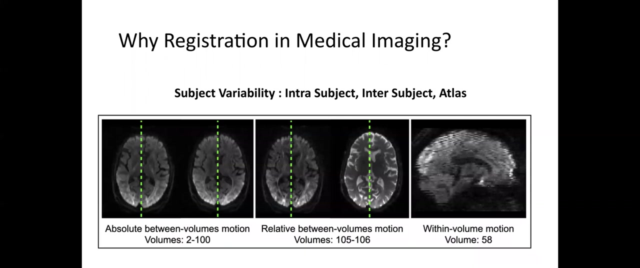 And to augment the information of your data. In our field, diffusion imaging, You will have to, under one of the most common and challenging scenario: The motion, The scan Children Or adult Patients. So in this illustration I mean indeed, a typical diffusion imaging dataset consists in n volumes. 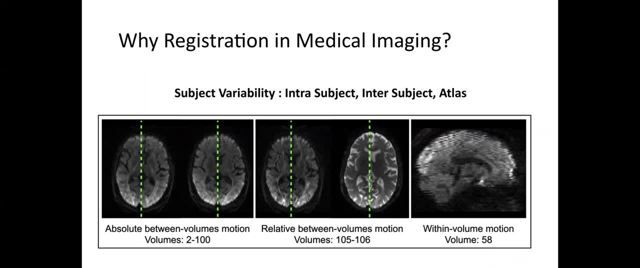 The voxel and densities of each volume reflect properties of the water molecule displacement along each of the sample diffusion encoding settings. Okay, So A motion between a volume is really frequent during a patient scan. So you can see in these four first images in this illustration. 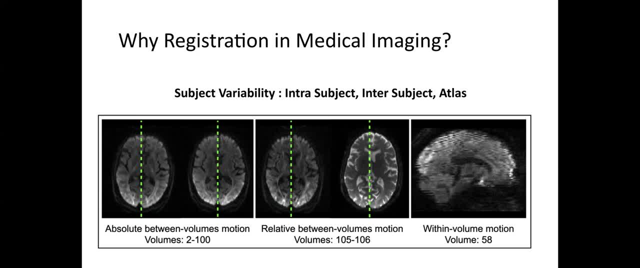 We represent this between volume motion. The last image on this illustration represents the within volume motion Meaning A significant Subject motion- between the acquisition of the first slice And the last slice of a single diffusion imaging volume. This last case We usually encounter it. 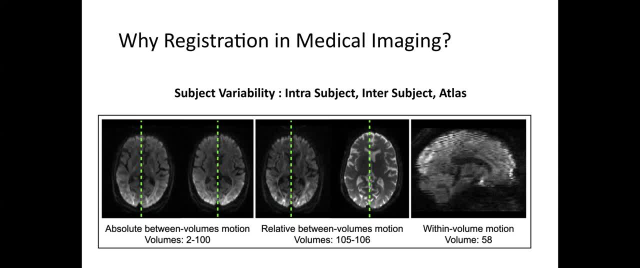 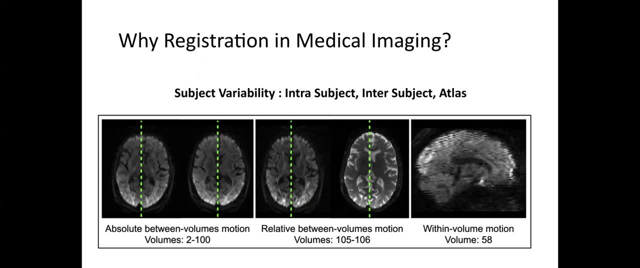 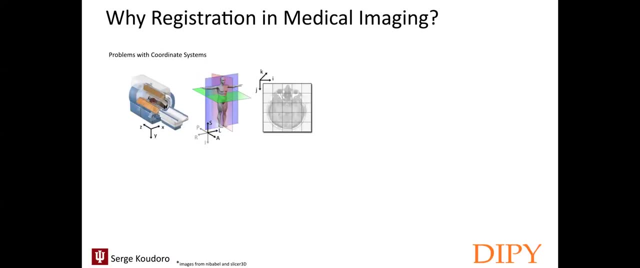 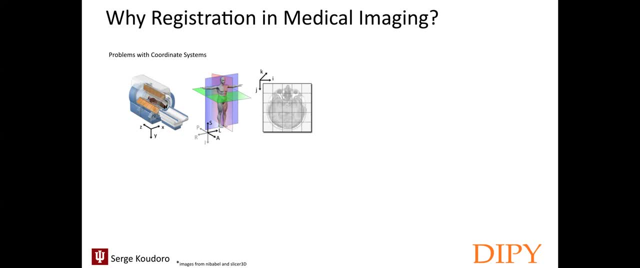 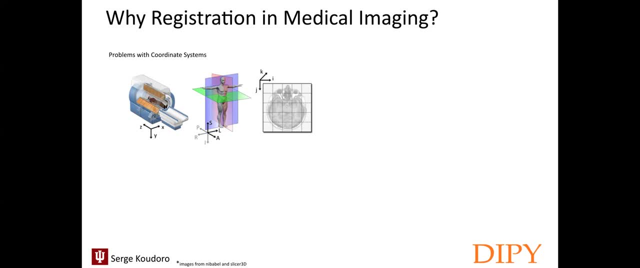 represented by anterior, posterior, right, left and inferior superior. An easy example is the neurologist and radiologist convention. As you can see in the picture here, the subject has a stroke in the left temporal lobe causing a dark area on the MRI scanner. 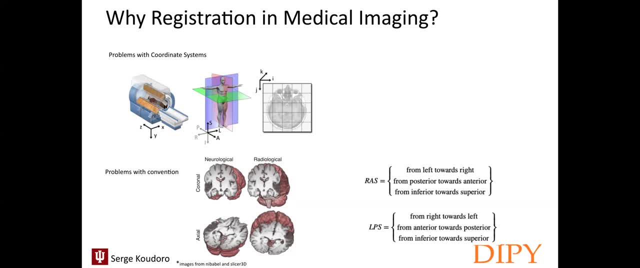 Are you sure? Are you sure Left or a radiologist can say, Because his coordinate system is quite different: we use LAS, which is in neurologist, we will use RAS, as you can see on this picture. Then the last coordinate system that you can see is IGK. 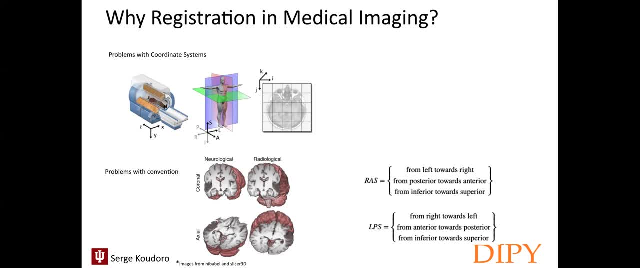 So this coordinate system is a is common for all the algorithms who work with a grid. When we project our object from the physical space to the grid, we certainly have a different size, scale, orientation and we need to normalize it. We want to make sure that we transform a different set of data into one coordinate system. 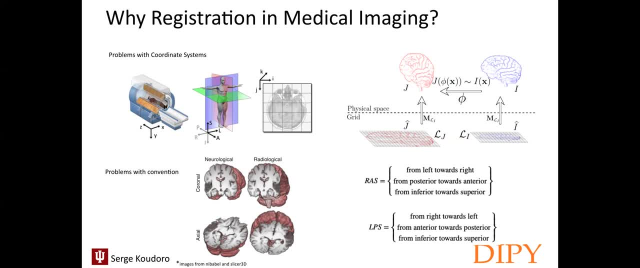 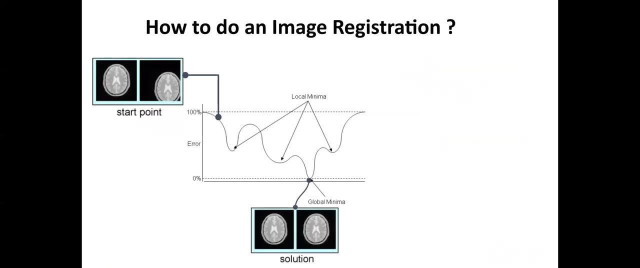 This transformation might imply some misalignment. So now let's briefly: how can we achieve this alignment? So how to do an image registration? Image registration at the end is an optimization problem. At the starting point you have a measure to compare two datasets. 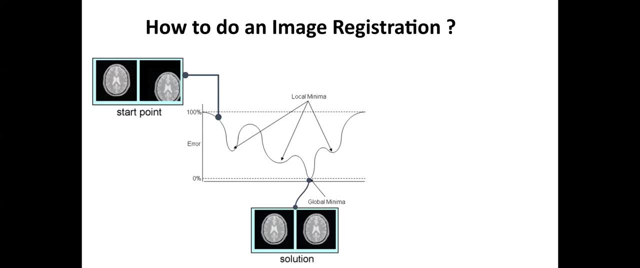 Of course, the two datasets should be in the same space. So here in this figure you have this point where the measures live in a specific domain. We want to minimize the difference between these two scans. If you have a small measure difference, it means that the alignment is closed. 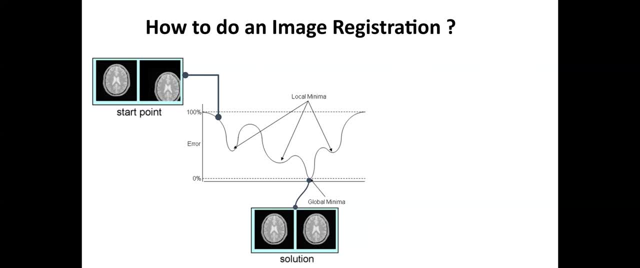 If the measure is bigger, of course, it means that we are going further and further between our two volumes. The challenge of the optimization is to find, in this high dimensional space, the global minimum of this measure, which is not a trivial problem. 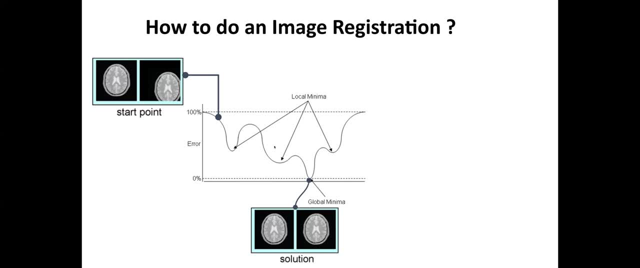 As you can see in this illustration, you can be easily stuck in a local minimum And the whole field is working on this optimization problem. Usually, a spatial normalization or a spatial transformation consists in three parts. So, as we said just before, the first part is picking the optimization method. 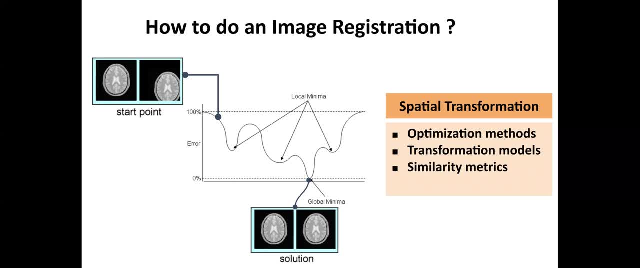 I will go further on the second video concerning this part. The second part is picking your transformation model, So which method you will use to align your two volumes, And then the similarity metric, which will give you a value to estimate how well are they aligned. 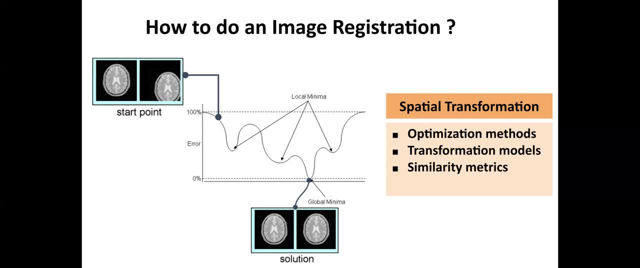 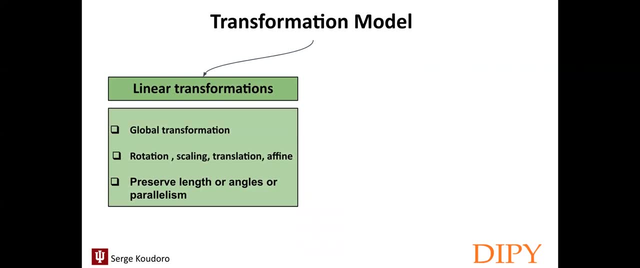 So let's have a quick overview of the transformation model. The transformation model can be divided into two categories: The linear transformation category with some specific features. Usually this is a global transformation. The linear transformation is composed with rotation scaling transformation. 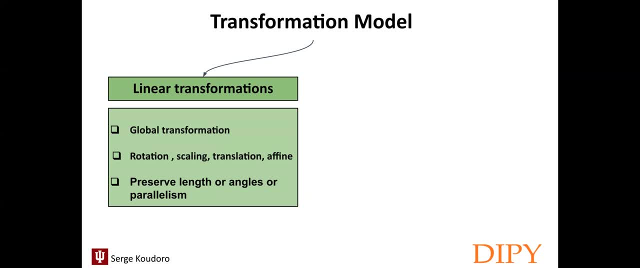 And I will go more in detail in the second video. But the most important part and feature that you need to keep in mind is the linear transformation. preserve length, angle and parallelism. The second category is a non-rigid or non-linear transformation. 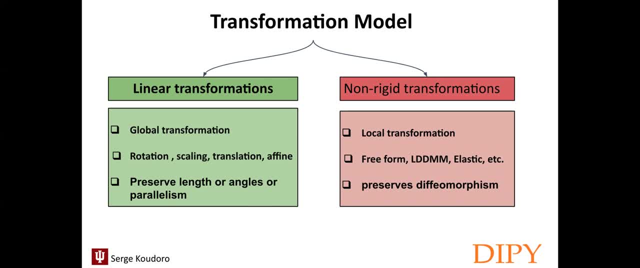 Which, in this case, now we are working more locally- We have a different technique, Like freeform, LDDMM, elastic- Same. I will talk more about it on the third video, And this time we don't preserve the parallelism, but we preserve the geomorphics. 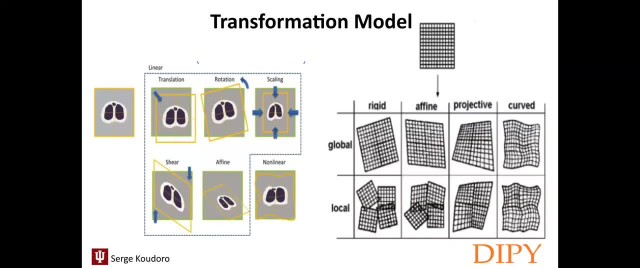 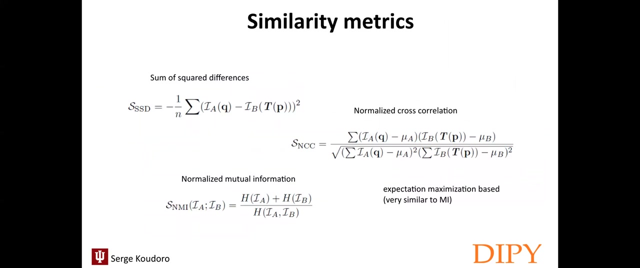 So to illustrate that you can see here, on the different figure, how the difference between working locally and globally, and what is it to preserve? The deform morphism or the parallelism? The second point is the similarity metric Metrics are probably the most critical element of a registration problem. 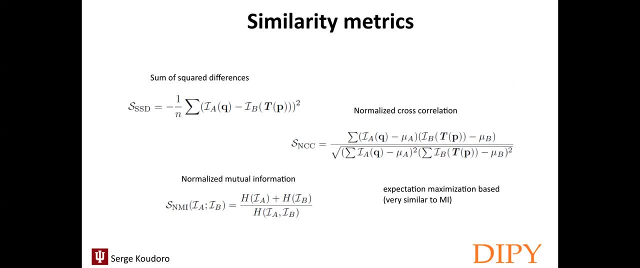 It quantifies the similarity between two volumes. They measure how well a target object is matched by the reference object after any transformer has been applied to it. The more the score is higher, the more similar are the volumes. If we think about it, it is a bit kind of the inverse of a distance metric. 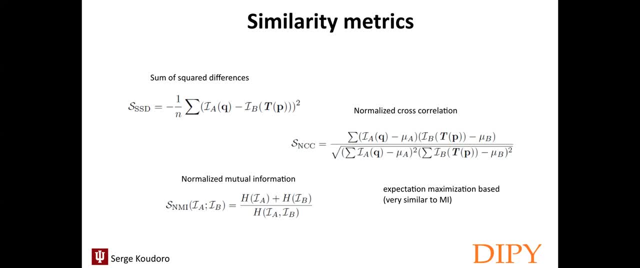 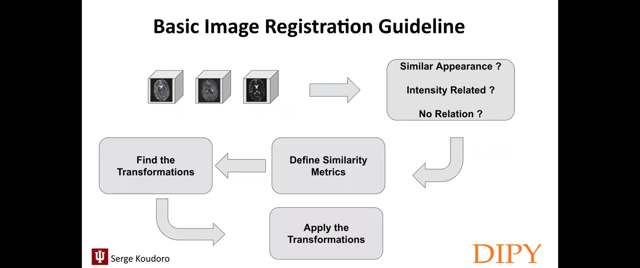 So how to choose them. This is a really complex and we will talk more about it on the part two, But to give you a small overview, you can see on this figure a global guideline on how to pick your metrics. So let's start with at the beginning. you have your volume here. 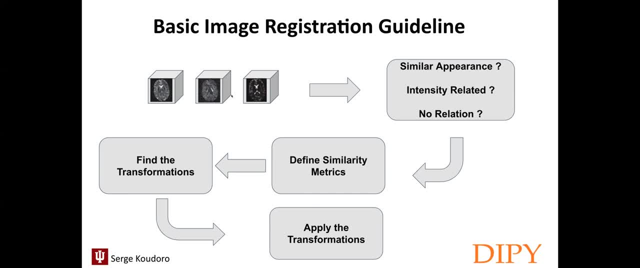 You want to check if they have a similar appearance. So this is really the first question that you have to ask yourself when you start to do an image resolution: How look my volume? Do they have a similar intensity? So by asking all these kinds of questions,